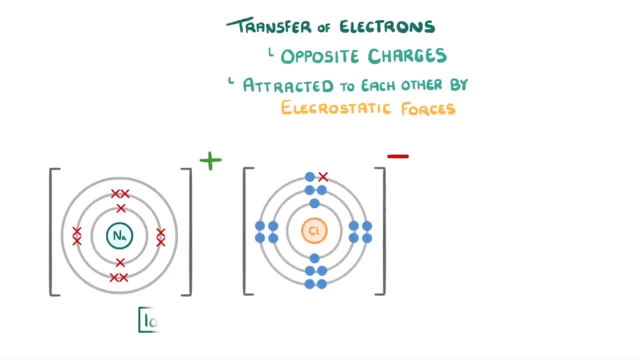 other by electrostatic forces to form an arnic compound. We call this force an arnic bond and it's really strong, similar in strength to covalent bonds, which we cover in another video. The way that we've drawn our compound here is known as a dot and cross diagram. 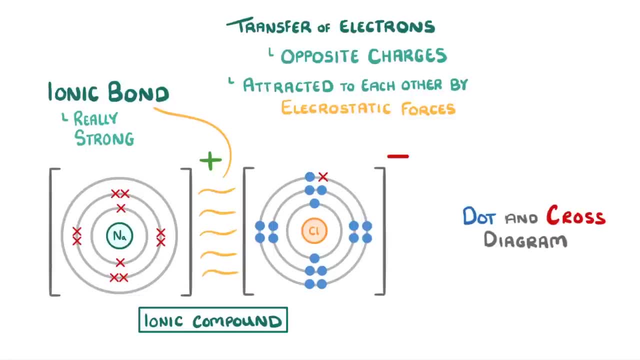 you'll often be asked to draw things this way in your exam To do it properly. there are a couple of features to notice, though. One is that we've drawn the electrons of one atom as dots and the other as crosses. This is so that we can. 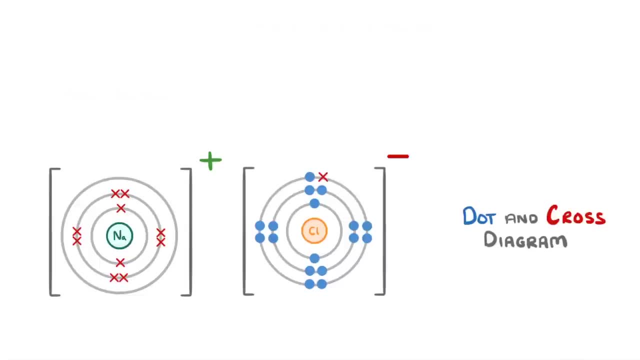 tell which electrons belong to which atom, And you should show the movement of any electrons with an arrow. Notice that in this dot and cross diagram, we've shown every electron shell of the atoms. Sometimes, though, you'll be told you only have to draw the outermost shell, which is a bit quicker to draw, and for our 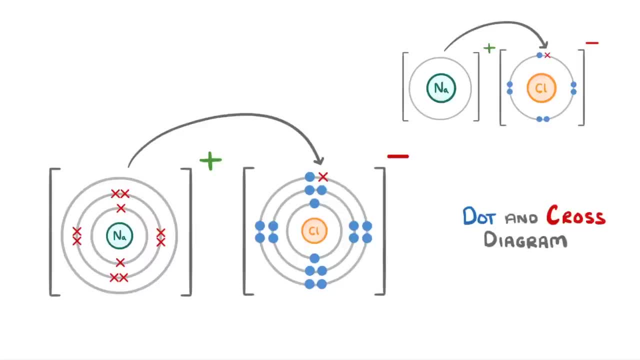 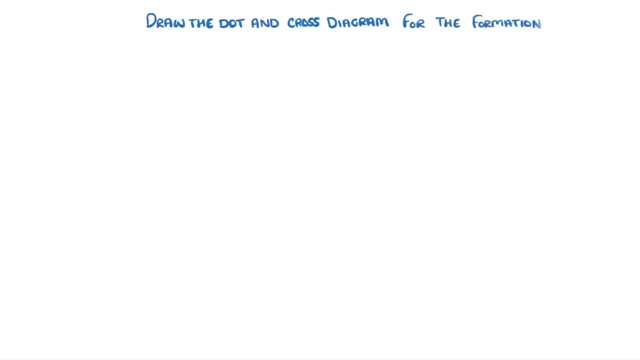 example, it would look like this: Let's consider a harder example. Draw the dot-and-cross diagram for the formation of magnesium chloride, MgCl2.. Only draw the outermost shells Now. this time we can see that we have three atoms in the compound rather than. 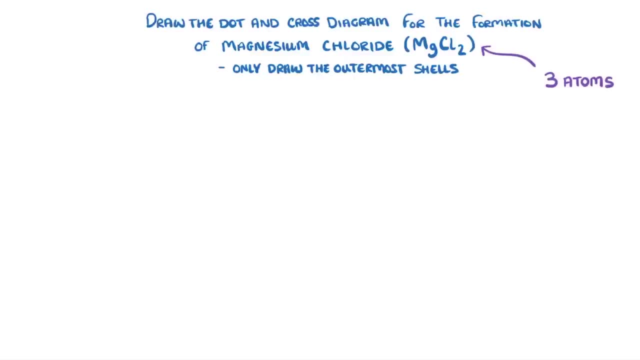 two. To start, let's draw this image out: our reactants. We have magnesium, which has two electrons in its outer shell that it wants to get rid of, and we have two chlorines, both of which have seven outer electrons, so we need one more each. The next step is to think about where the electrons could move. 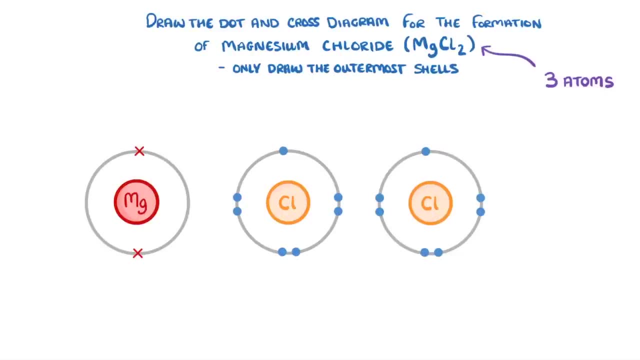 to make all the electrons happy with a full outer shell And, as a general rule, electrons will move from the metal to the nonmetal, So in this case, magnesium can give one electron to each of the two chlorines. As a result, we'll end up with a magnesium 2 plus ion. 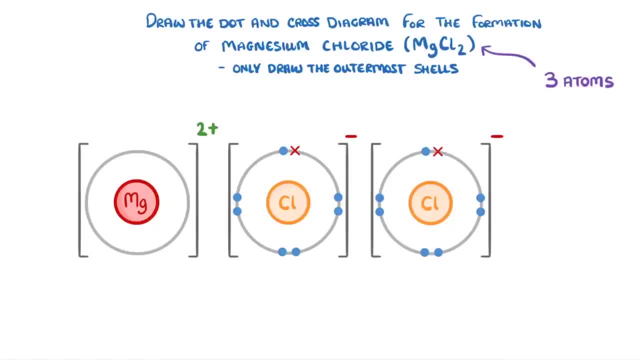 and two chloride, 1 minus ions. This is now pretty much done. however, in dot and cross diagrams involving more than two ions, we generally arrange the ions like they would be arranged in a real compound. So because the chlorides will both be attracted to the 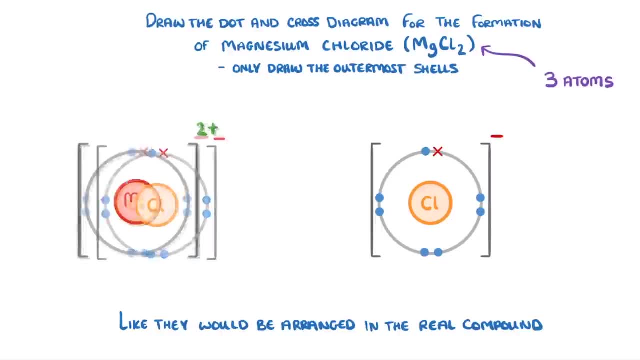 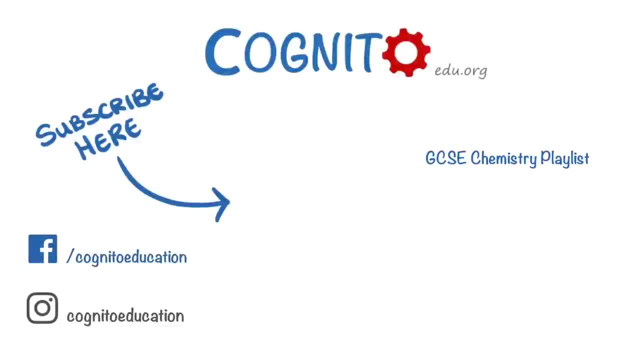 positive magnesium. we place them on either side of it, And that's it for this video. If you enjoyed it, then do share it with your friends and we'll see you next time.